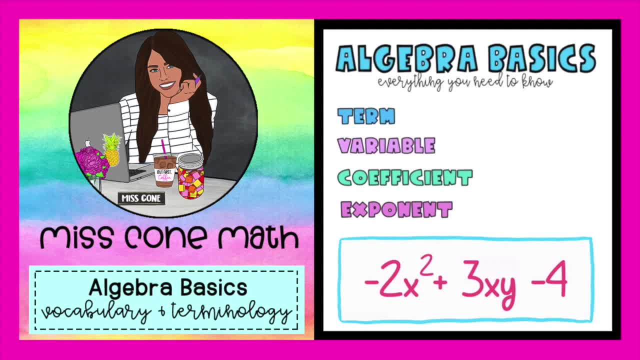 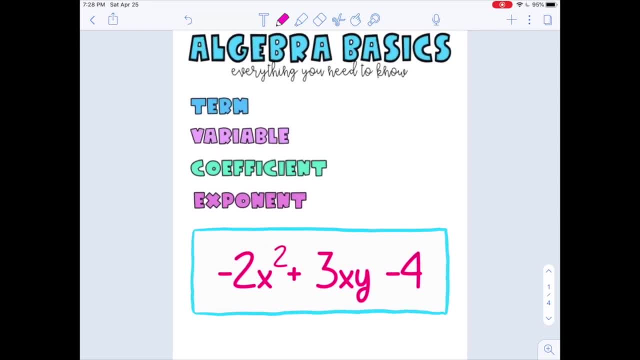 So in this video I'm just going to go over some of our algebra basics, some terms that we're going to be using non-stop. The first is- term- That makes sense, right- Variable, coefficient and exponent. You guys already know what exponents are. We went over them earlier in the year. 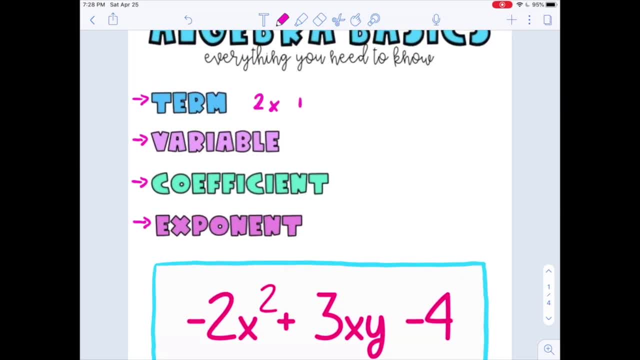 but this is just a little review. I also have a problem below that I'm going to be referencing. A term is any number or variable that can be added or subtracted. So 2x is a term, 4 is a term. 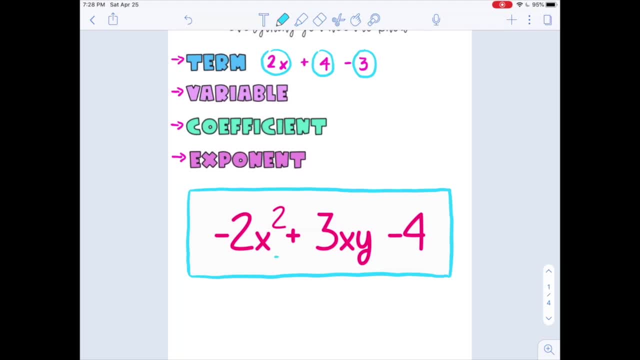 3 is a term. So if you look below all of those separate entities, so you have negative 2x to the second power. that's a term. 3xy is a term. 4 is a term. They're separated by a plus and a minus. 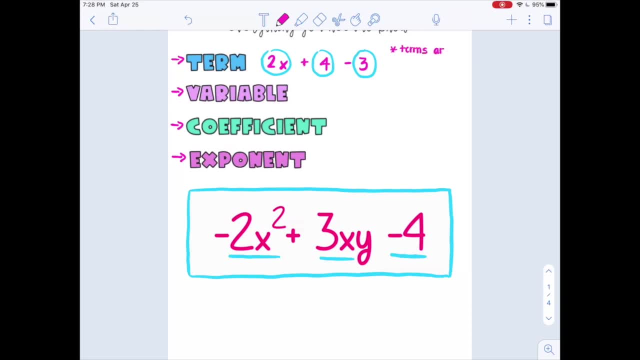 Sorry, I just like stuttered there. A plus and a minus, So terms can be large. Sometimes you'll get something that is very long, but as long as it can be, it is separated when you look at it by a plus or a minus, it can still be a term. Moving on to variable, we kind of went over this. 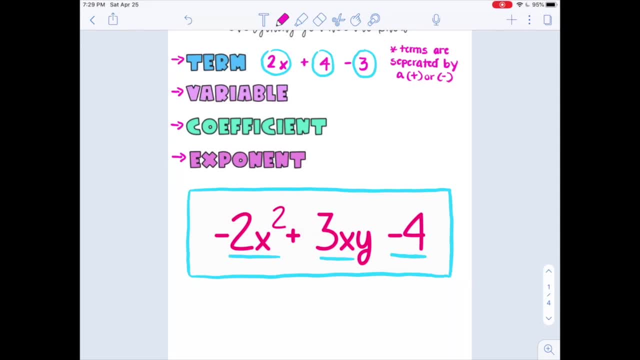 right before vacation. but a variable is basically your x, your y, z, any letter that can be used to represent an unknown number. So in this case, we don't know what x equals, so we're just going to use x as a placeholder. Same thing for y. Whenever you see a letter. 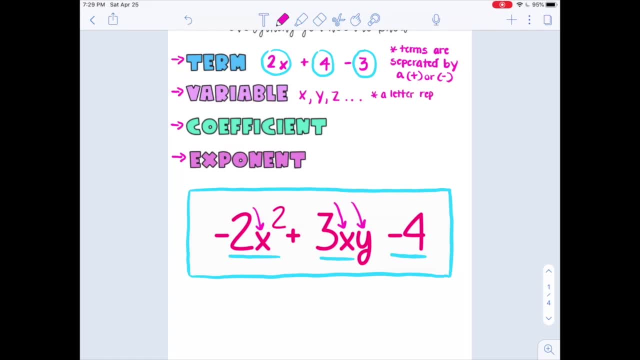 you think boom variable. Okay, so it's a letter that is representing a number that we don't know yet and we are probably going to try and figure it out at some point. We're not quite there yet, but that's the goal. typically in algebra is to solve for an unknown number. So if you're 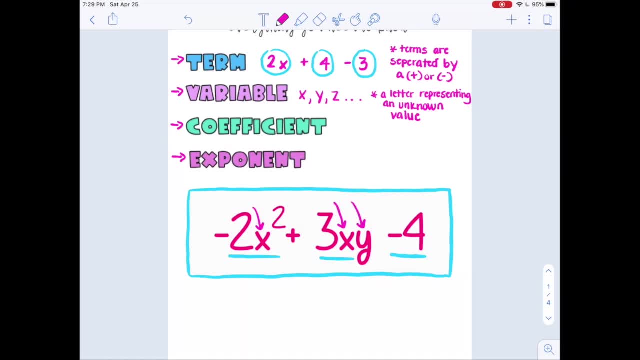 going to solve for an unknown number. okay, coefficient. this is where it's going to get a little tricky, but I think you guys can handle it. The coefficient is the number that is in front of a variable. So if you look below, we've got an x and then we've got a negative two in front of.